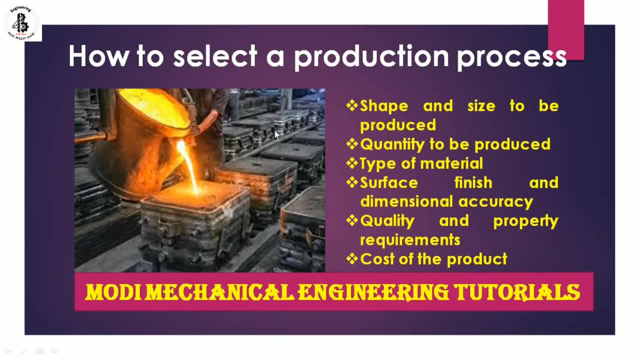 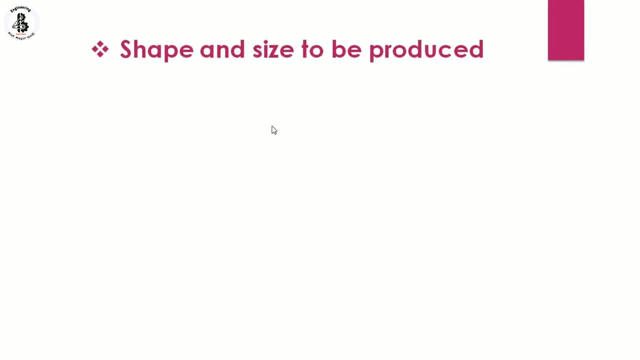 be the some of the fundamental discussions on to these theories. So let us start with the detail explanation. So, first of all, starting with the shape and size to be produced, So, in that case, for products with a simple shape, So that will be the best suitable production process and that will 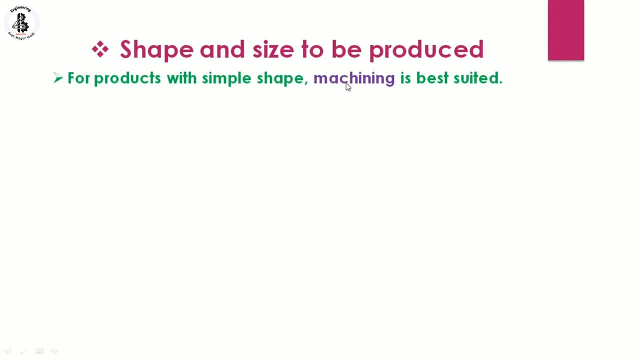 be machining So by the unwanted removal of the materials from the raw materials and that will be converting into the desired shape and size. So that will be the best suited method As a production method and that would be considering as a machining Then for the complex. 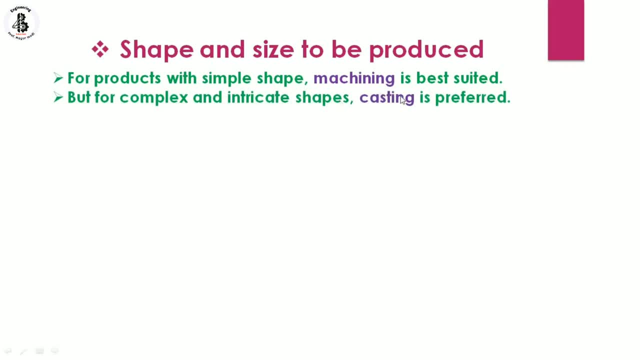 and integrated shapes. So at that time it will be casting is to be preferred. So casting, that will be also the fundamental manufacturing process, or you can say production process that will be used to manufactured, to complex and integrated shapes. So such kind of shapes that will be having a 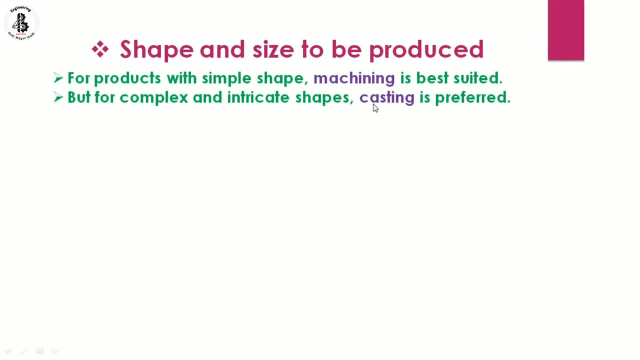 difficulties to machines. so that's why we are most preferring methodology and that will be casting then. the size of the product is also an important factor. so, as per the requirements of the applications, the size of the product, if it will be the extremely small size. so that will be the some another manufacturing. 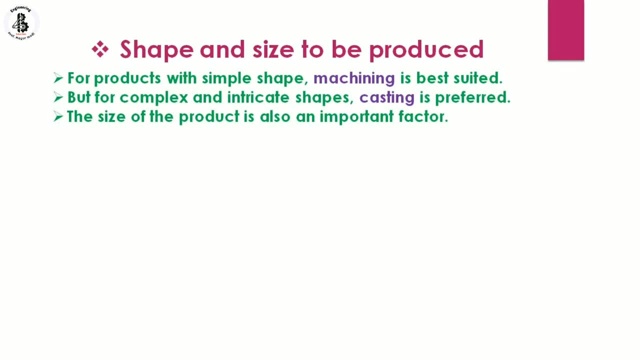 process. if it will be the large size of the components, so it will be the another manufacturing process, so as per the requirements of the size of the products, it will be having a different kind of production processes. then just you can see here it will be the one example long product such as. 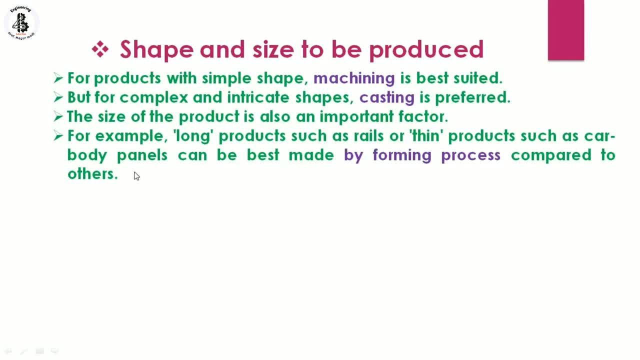 rails, or you can say thin product, such as car body panels, so can be based, made by a farming process as compared to the other process. so basically in a production process, the starting with the machining process. so that will be considering as all the cutting process and that will be. 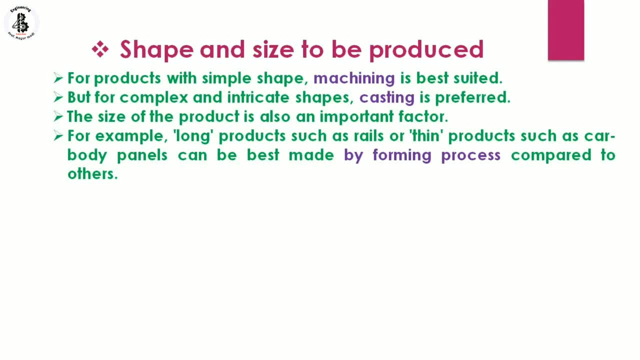 conventional cutting, or you can say non-conventional cuttings, or you can say advanced cutting processes. then you should also use some of the casting process, which will be having a big size of the components, as well as some integrated shapes that will be easily manufactured. then you can also use a powder metallurgy process and you can also use a. 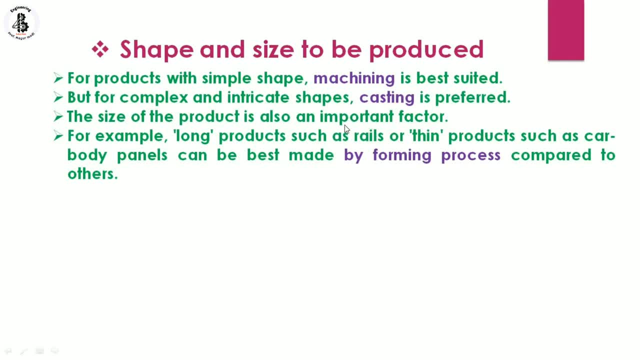 foil forming process, or you can say shape changing processes. so basically that will be the first, that will be known as a shape and size to be produced. so that will be the one of the factors for a selection of the production processes. then second, one quantity to be produced. so 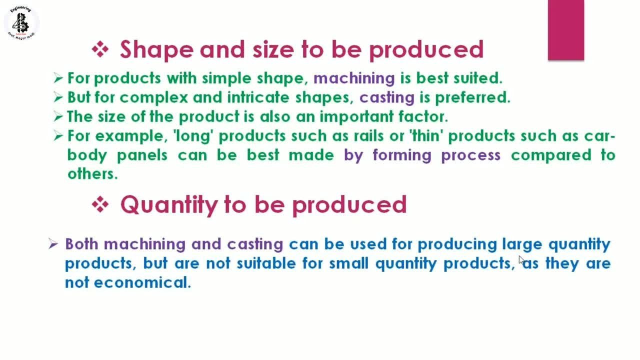 both the machining and the castings can be used for producing large quantity of the products, but are not suitable for the small quantity of the production process. so that will be the one of the products, as they are not economical. so in case of the machining and castings- or you can also add- 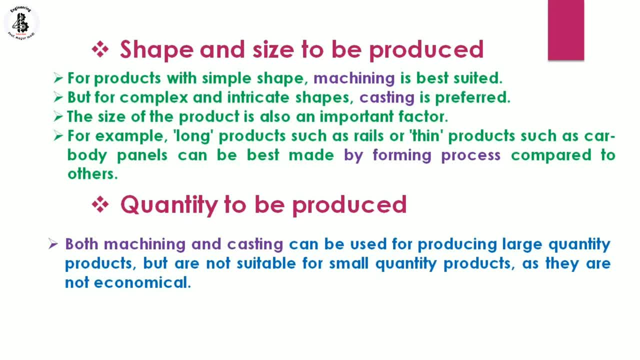 a powder metallurgy process which is having a good production, and that will be only feasible with respect to the economical consideration for only for a mass production. so if it will be the number of quantities, it will be into the larger size then and then it will be having a good 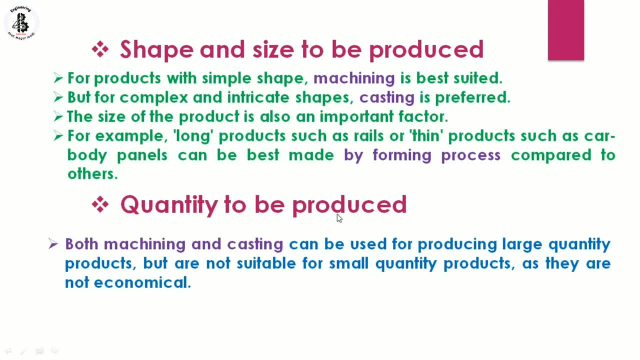 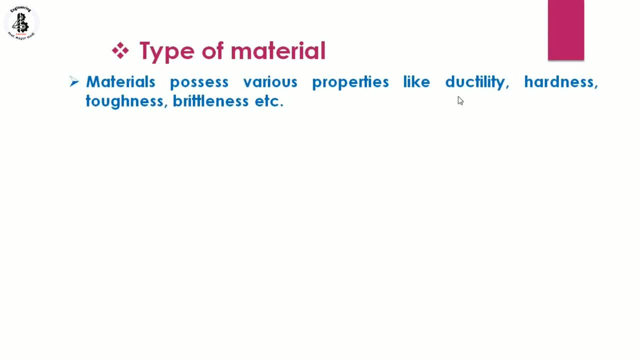 feasibility. so second one, that will be quantity to be produced. so that will be the one of the factors for a selection of the production processes. then, third, type of materials, so material processes, various properties like ductility, hardness, toughness, brittleness, etc. so which kind of material is being selected for a workpiece materials? according to that it will be converting. 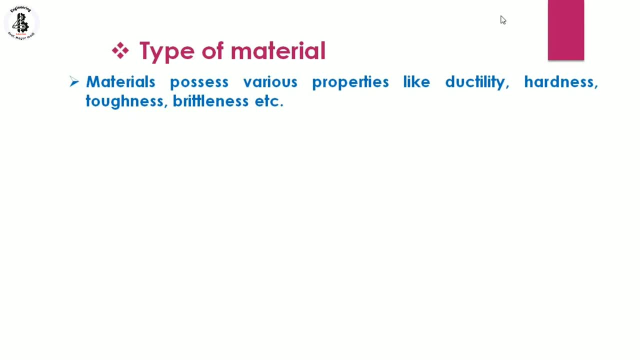 into desired shape and size. so as per the selection of the materials, that will be selection of the production processes. So the hard materials cannot be machined easily, so you should go for a powder metallurgy process, or you can say you can also use a casting process to manufacturing of the such kind of components. 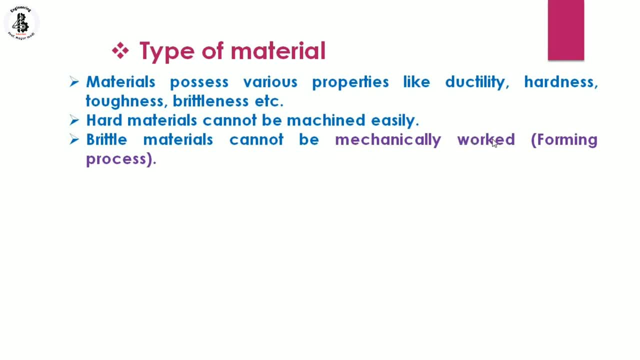 so brittle materials cannot be mechanically work or you can say that will be not, forming process is being used because that will be the least ductility. so at that time for the brittle materials you should preferring a casting, or you can say: most preferable that will be the powder. 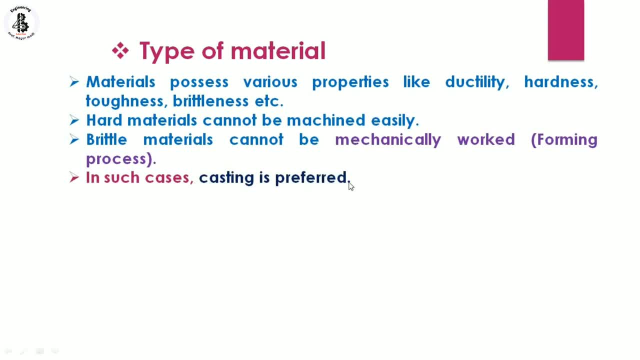 metallurgy. In such cases casting is being preferred, or you can also use the powder metallurgy process for a brittle materials, so that will be also having a good mechanical properties. then surface finish and dimensional accuracy, so such kind of things. according to the dimensional accuracy, that will 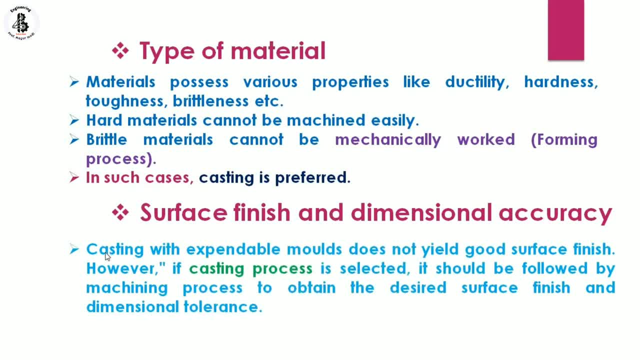 be the requirements as per the shape and size. so you need to control that. so, for that, casting with expandable molds does not yield good surface finish. So, however, if casting process is being selected, so it should be followed by machining process to obtain a desired surface finish as well as the dimensional tolerance. so, after the casting process, 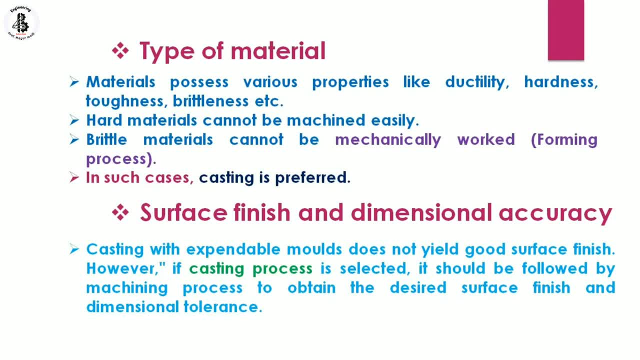 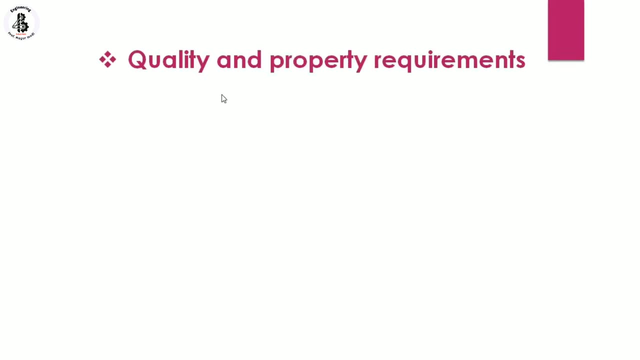 there will be the requirement of the secondary operations, or you can say some of the machining operations for increasing the surface finish, as well as the dimensional accuracy. so as from the requirement of the surface finish and dimensional accuracy you should select a such kind of process, then quality and property requirements. so basically a defect-free product with specific 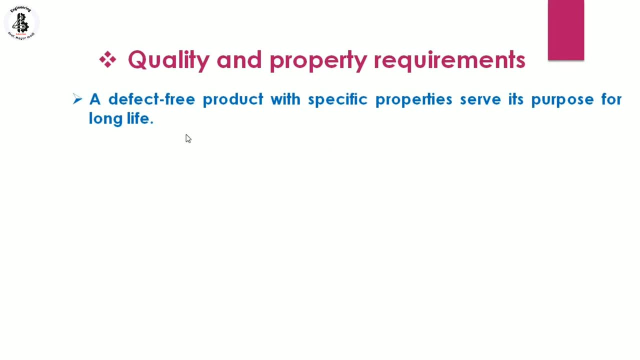 properties, so its purpose, for a long life. so that will be the essential requirement of the any production house. so properties of the cast materials are generally less when compared to that a mechanically work materials. so in that case of that casting process or you can say cast materials, 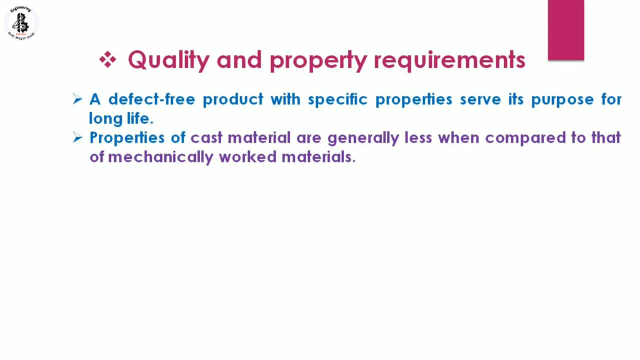 so that will be having a less escalating process. Also, the manufacturing process will be selected like in production house, so that will be a lot of defects compared to the mechanically work. So, as per the my requirements of the application wise, i would like to select such kind of production. 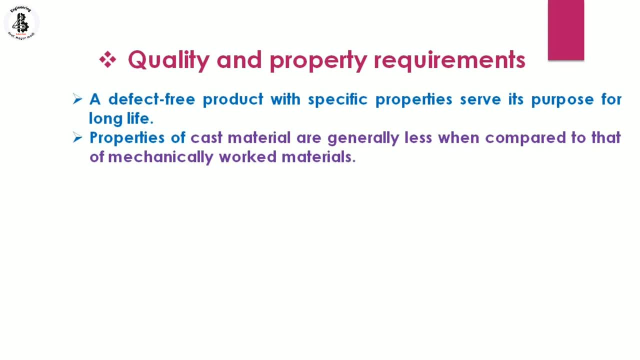 process. so which will be preferable as for the economic conservation as well as the durability of the product. So without compromising with the quality of the products and that will be into the minimum cost, such kind of production house, or you can say production processes, is being selected. 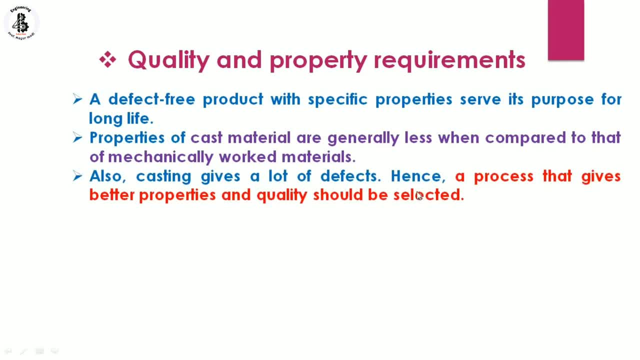 that gives better properties and quality should be selected, As we already discussing on that, without compromising with the quality. you should go for a economical production processes. Then last one, an important one: cost of the product. so customers often demand for the products with more features and the performance at a reduced price. so that will be the always you should go.